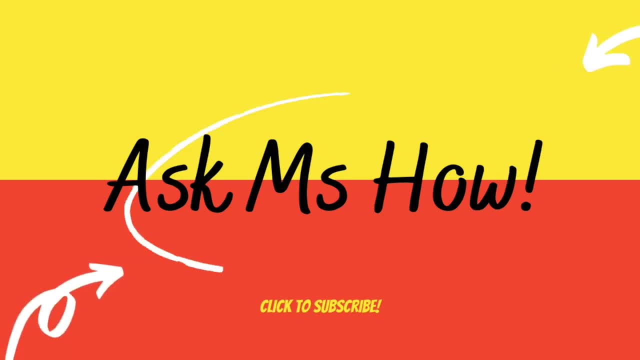 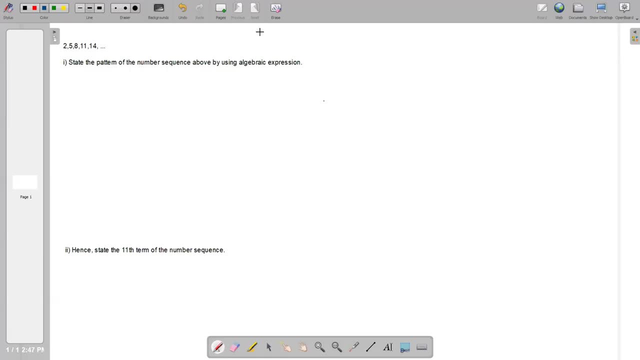 Hi class, so I see you again. So today we will learn how to form algebraic expressions. or sometimes the questions will name it as find the anthem. So most of the time students not sure how to find when the sequence numbers is given like this. So first thing, okay, when we want to. 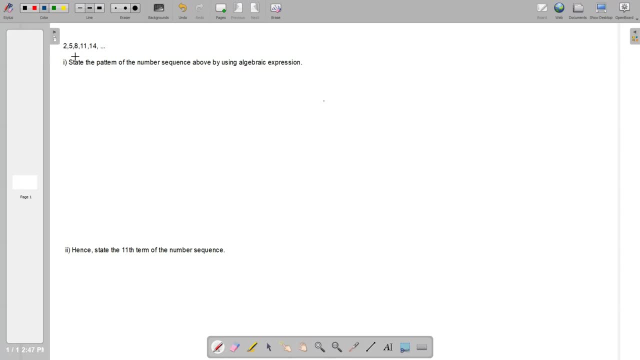 find the pattern of the number sequence. So first what we can do is to find the difference of each number, So 2 to 5, the difference by 3, 5 to 8, also 3, 8 to 11, also 3, 11 to 14 is also 3.. So we can. 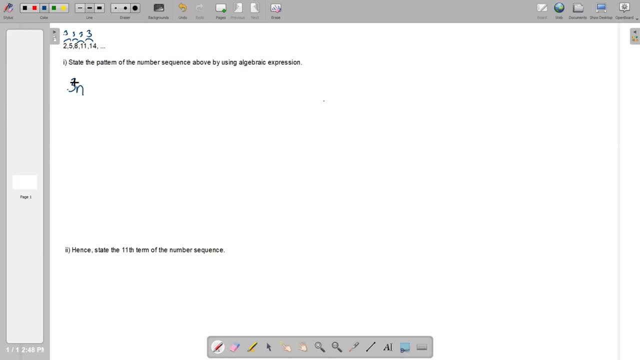 start with okay, 3n, Okay. so after that, okay, after that, okay, we will need to try. if, let's say, our anthem is 3n, Okay, let us try. So when your n, your n, equals to 1, since your anthem is 3n, we try. 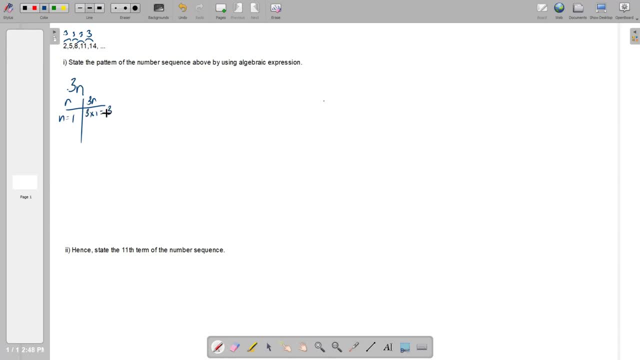 So 3 times 1, you get 3.. So class now let us look at here. your 3 is not the same as the 1 given here, which is 2.. So from 3 you need to get to 2 what we need to do, So 3. 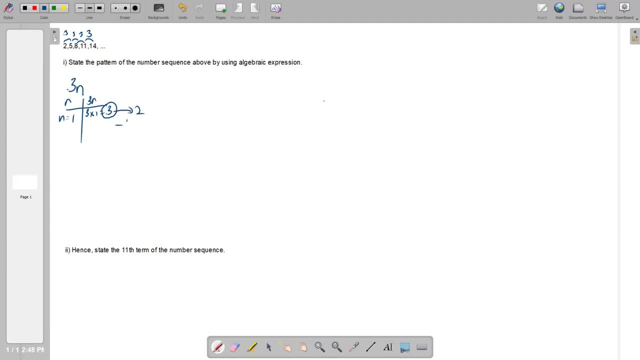 you need to get to 2 with minus 1.. So meaning to say that 3n. okay, we have to do some adjustment. So instead of getting this 3n now, let us our 3, our anthem, become 3n minus 1.. So then we need to test whether this formula is correct or not, Which each of the 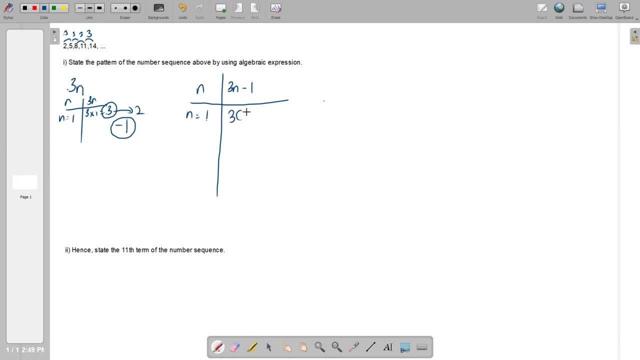 terms. so we have n equals to 1.. So 3 times 1 minus 1.. So we have 3 minus 1, we get 2.. So class bear in mind we have to check with the after every term. so that is the we see. 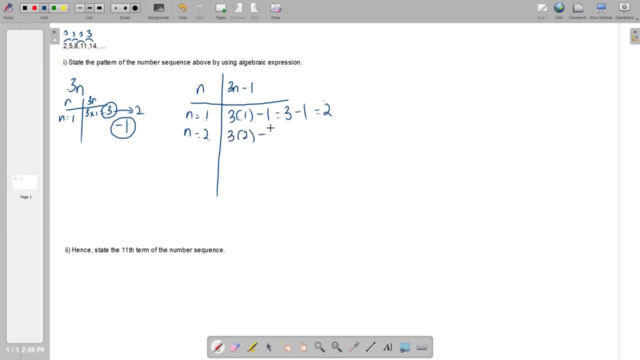 is the same. so 3 times 2 minus 1, so we have 6 minus 1 equals to, okay, 5, and next n equals to 3. so 3 times 3 minus 1, so 9 minus 1, we get n, and then n equals to 4. 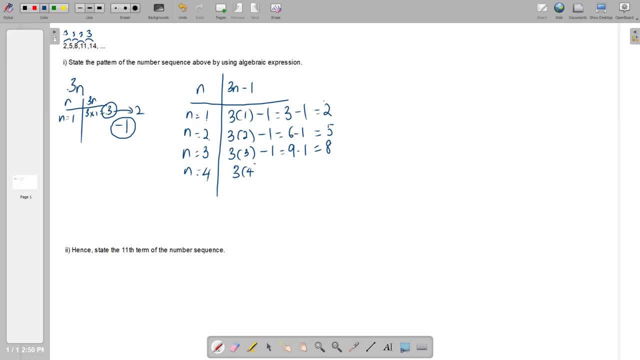 okay, 3 times 4 minus 1, so we have 12 minus 1, we get 11. so n equals to 5. so 3 times 5 minus 1, we get 15 minus 1, we get 14. so now let us compare with the. 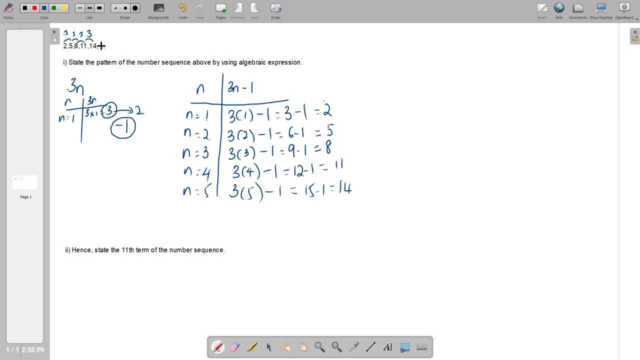 sequence that was given: 2, 5,, 8,, 11,, 14. and what we count 2,, 5,, 8,, 11,, 14. so meaning to say our algebraic expression is correct. so now we can form our algebraic expression. so 3 times n equals to 3 and minus 1. 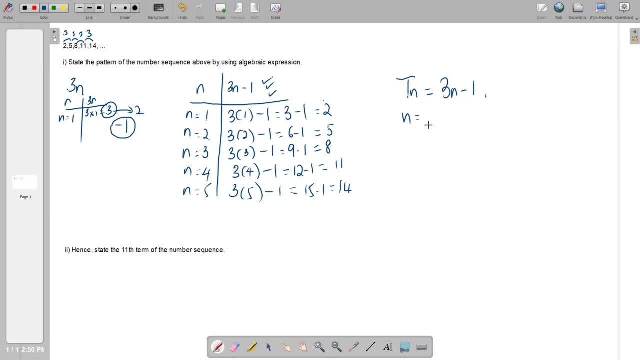 and what is your n? from 1 to 5. so we list up here. okay, so we list up to 5 is enough. so here, this is how we get our algebraic expression operations. So once we get our algebraic expressions, let us move on to the next. 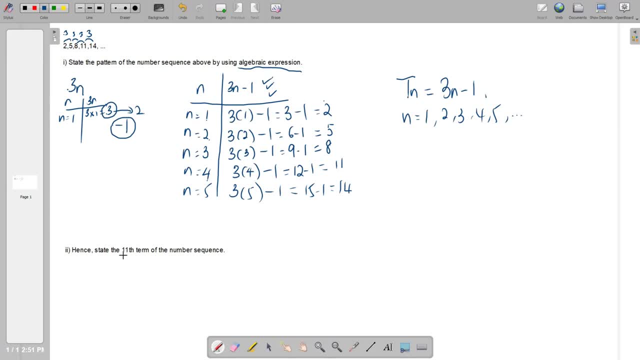 questions. Okay, this is a kind of equations that you normally get. First they ask you to form algebraic expressions. Next they ask you to find the sequence. So we look at 11 terms. So 11 terms mean t11.. So what we need to do is just substitute. So just now your n okay. 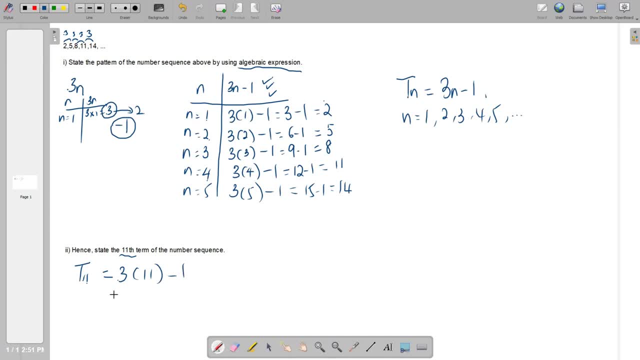 will become 11 now. Okay, so 33 minus 1, so we get a 32.. All right, so class. that's all for today class. So if let's say any of you you need extra explanations, okay, you need guide. 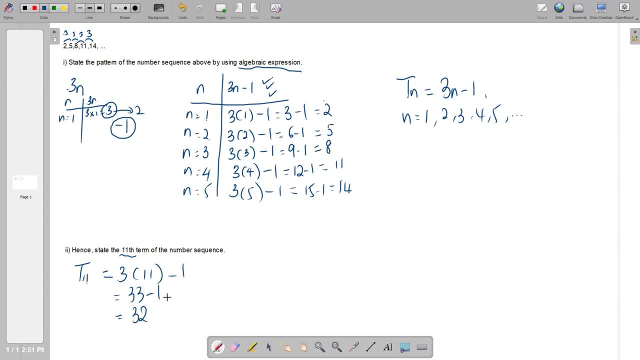 you need help or homework help, you can always contact me. So drop your comment in the comment box below or contact me through my email so I can guide you even better. Okay, so, I'll see you in the next video, So bye, bye. 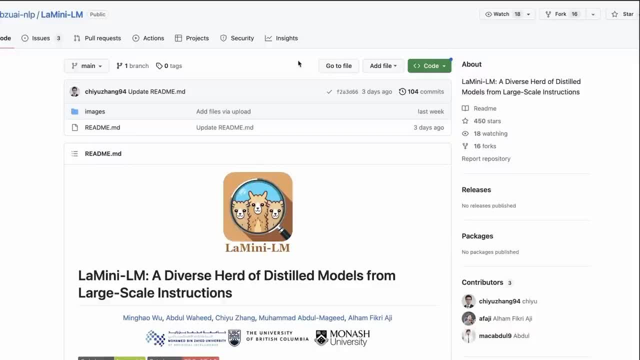 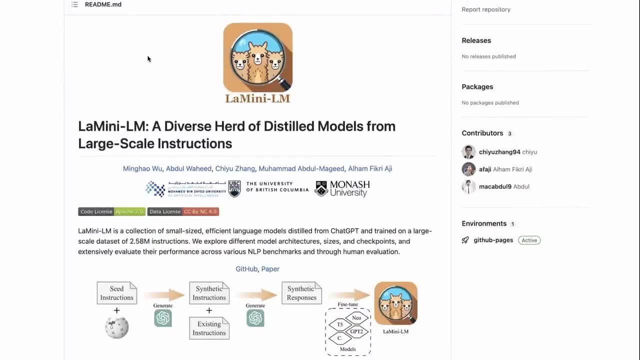 Okay, in this video I'm going to look at Lamini LM, a diverse herd of distilled models from large scale instructions. So this is based on a paper, but they've also released a code for this and 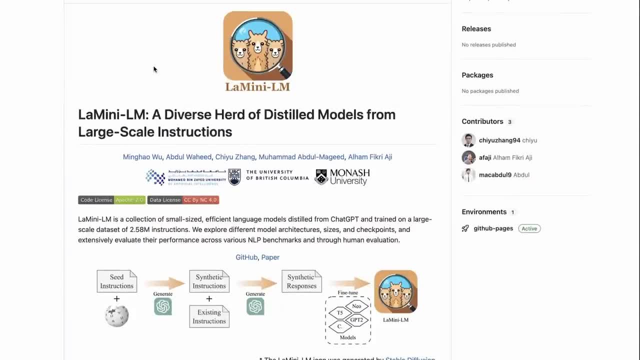 they've released a data set for this. I will preface this video at the start that if you're just here to find out if this is the latest best large language model, this is not the latest best 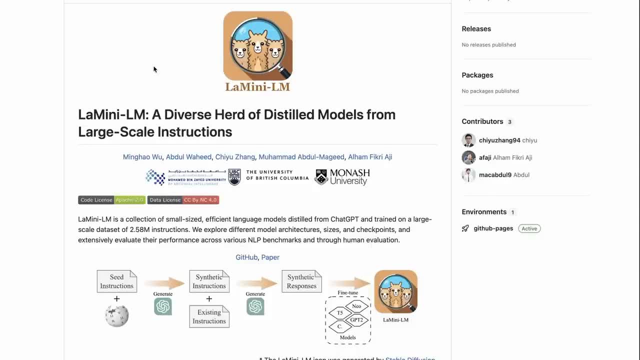 large language model. In fact, all these models are very tiny by design. And so if you're just here for that, this is probably not the video for you. Okay. But this is a super interesting paper 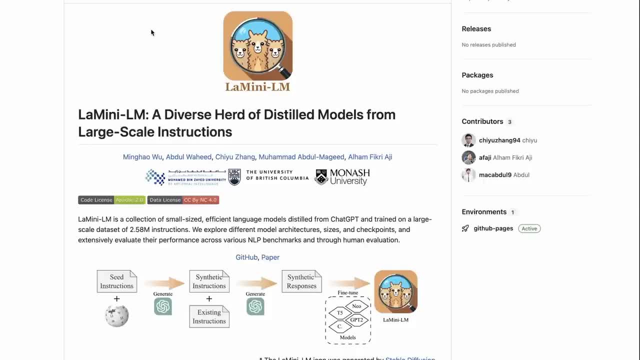 and a super interesting project. So I definitely want to sort of cover it and have a look at some of the things that they raise. And then also we'll have a look at the models and we'll have a look at 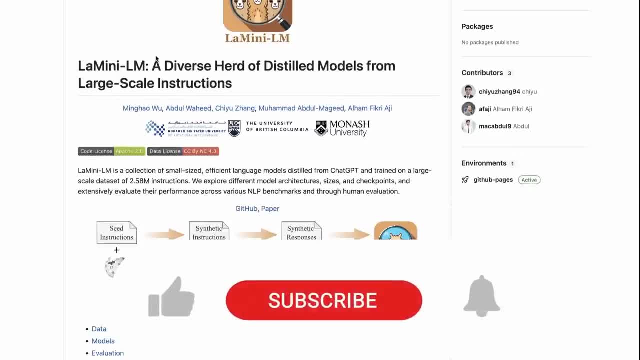 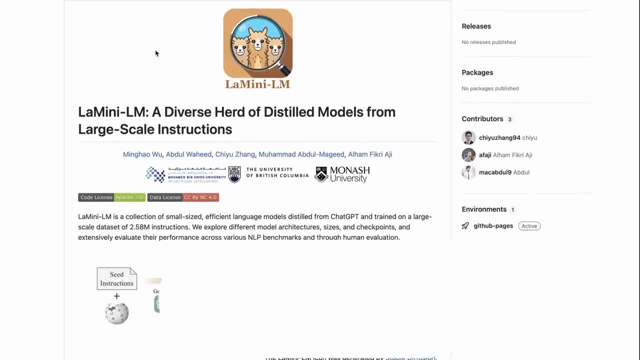 some of the code and stuff behind it as well. So the key idea here is that what they're basically trying out is that, okay, what happens if you go for a really small model, but you use a lot more scaled instructions. 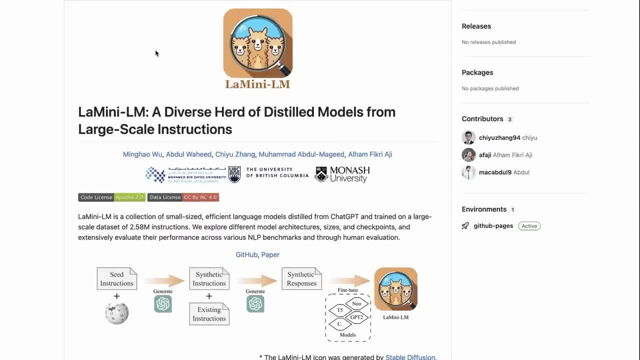 So if you think back to alpaca, alpaca only had like 52,000 instructions. The base model llama was a very large model. That was a 7 billion parameter model. But the number of instructions for alpaca itself were actually very small. So the idea here is to do the inverse of that, 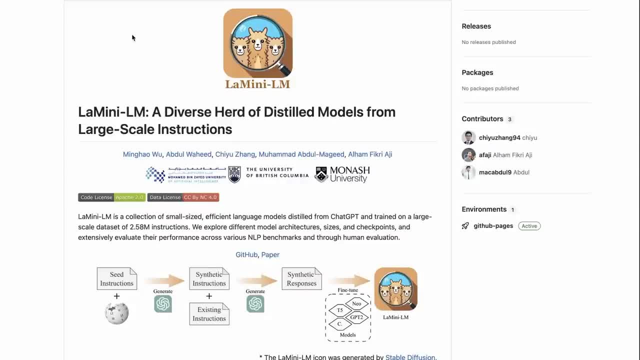 of go for a small model, but with a lot of distilled instructions. So, okay. What are they actually doing here? If we look at this diagram, we can sort of see that basically they've got some seed instructions. They then use a 3.5 turbo API to generate synthetic instructions and add those. And then they generate synthetic responses to these and their data set gets really big. So they've released the data set here and they've gone right